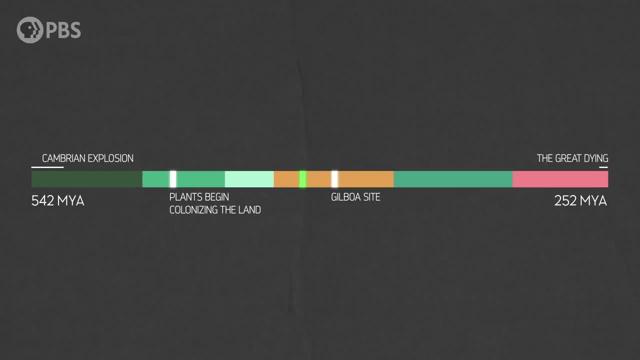 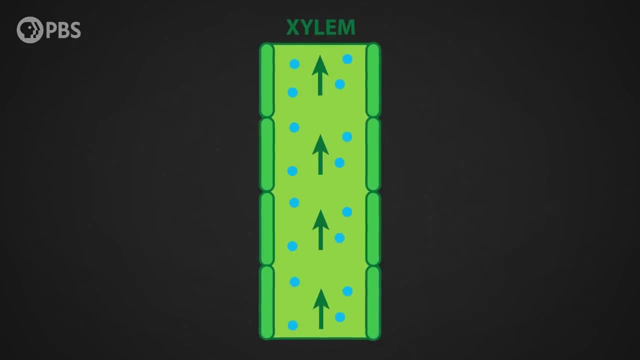 to 407 million years ago, almost 20 million years older than the woody plants of the Gilboa forest. By this time, many plants had developed a kind of vascular tissue called xylem. This helped move water from the bottom to the top of the plant. 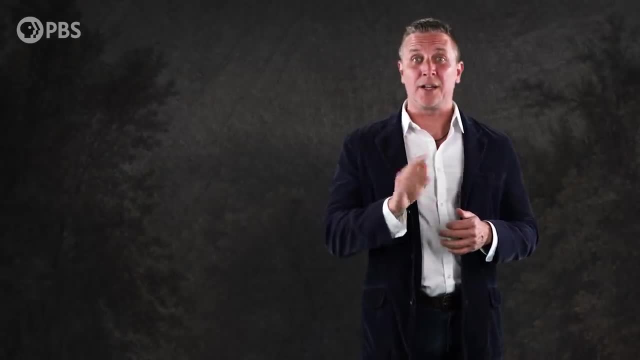 And pro tip: xylem is one of my favorite Scrabble words. If you play it right, you're looking at like 30 points at least, But that's not all. That new species of plant had more than one layer of xylem. 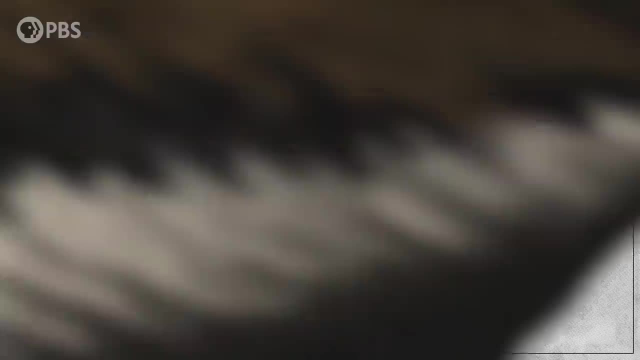 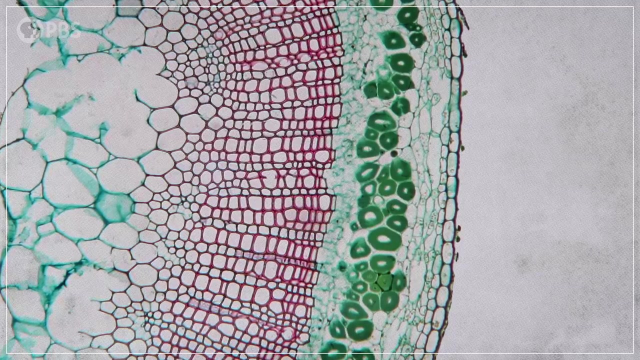 It had what's called secondary xylem, also known as wood Wood, consists of cellulose fibers and a compound called lignin, an organic polymer. Lignin and cellulose are major components of the cell walls of land plants, giving them structure and support. 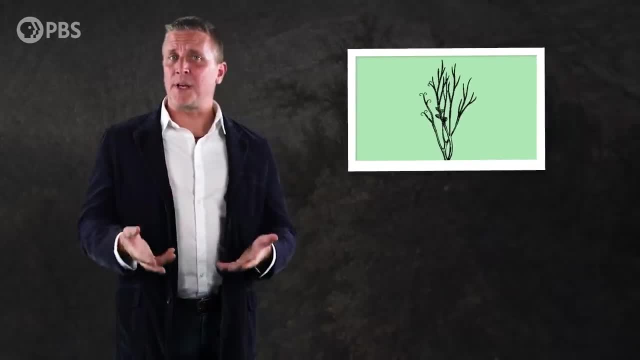 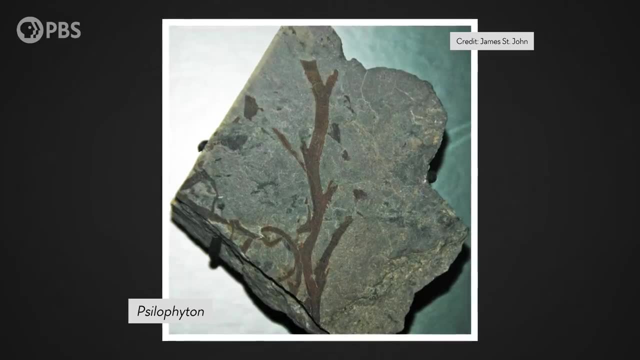 And together they're what makes wood so tough. Although these plants would probably have grown just a little higher than your ankles, they still spent energy on creating wood-like structures. So if these plants were so small, then why bother with wood at all? Well, probably to keep from getting thirsty. The earliest wood seems to have been a mechanism for transporting water more effectively than one layer of xylem could on its own, Because at this point in the Devonian, holding onto water was a real challenge. 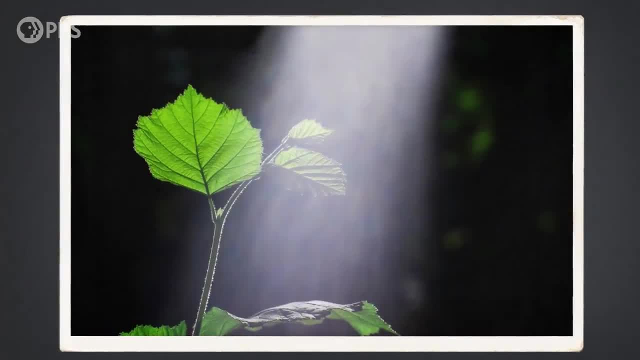 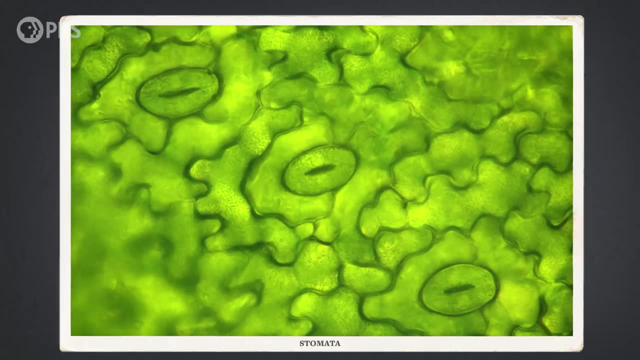 Stop me if you've heard this before, but plants need water, sunlight and carbon dioxide in order to photosynthesize And they absorb that carbon dioxide through pores called stomata. But those pores also allow for the evaporation of water And in the early Devonian the concentration of carbon dioxide in the atmosphere was going down. So plants needed to keep their stomata open for longer to absorb all the CO2 that they needed, And with those pores open longer, more water could escape. The development of wood was becoming an excellent strategy for keeping the whole plant hydrated, because it's really good at conducting water. So woody tissue seems to have first appeared as an adaptation for keeping plants hydrated. But plants didn't stop there. It's now thought that wood evolved at least five different times across different plant families by the late Devonian. It's a pretty clear case of convergent evolution. 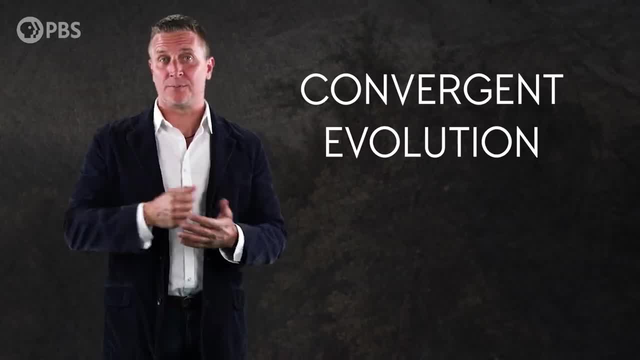 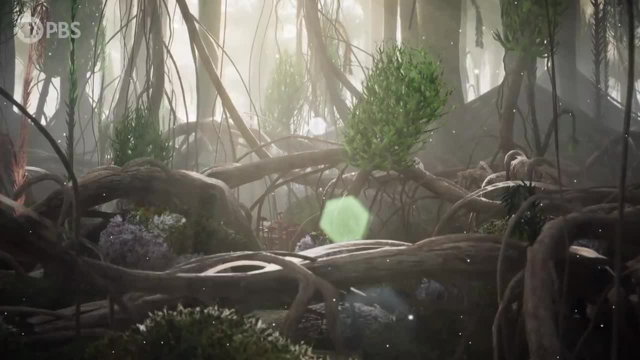 And as more plants developed the structure, they started exploiting new niches. Woody roots helped plants anchor themselves more solidly into the earth and allowed them to grow taller, And at the same time that plants were developing woody tissues, they were also making a few more modifications. When early plants first came onto land, most of them reproduced by releasing spores. This meant that they were really dependent on a wet environment. Otherwise the spores would fail to grow. The different reproductive cells they contained needed a thin layer of water. 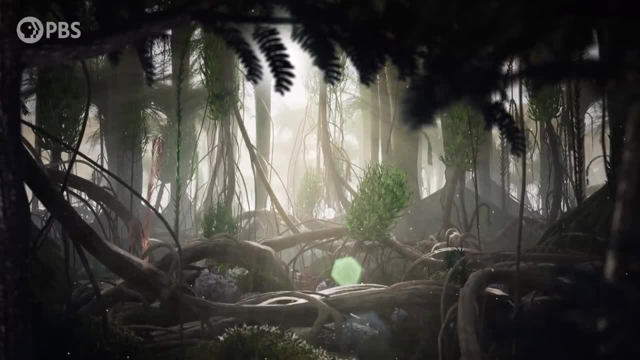 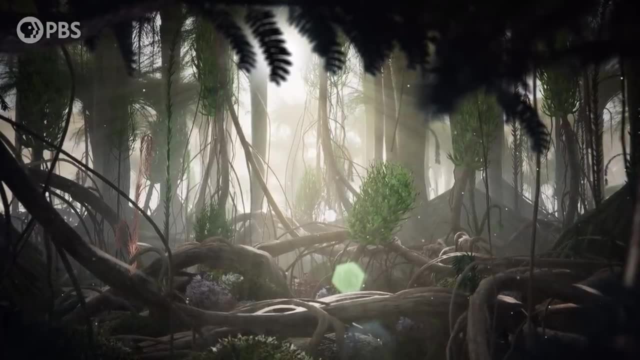 on the plant's surface to move around and come together. But once wood was around to help plants stay hydrated, some plants didn't need to rely quite so much on wet landscapes And they began developing different ways to reproduce. Take, for example, that plant I mentioned earlier, Archaeopteris from the late Devonian. 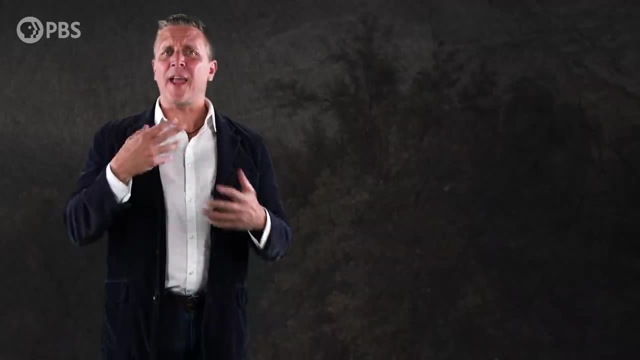 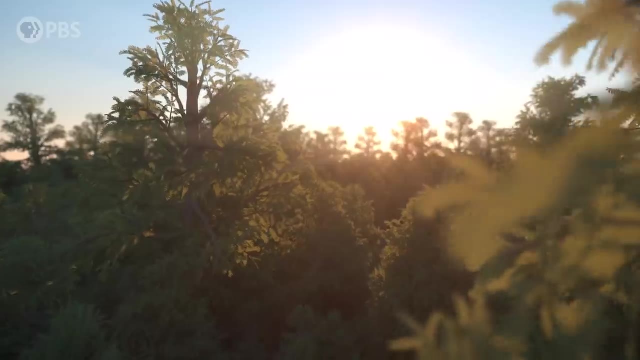 Its name means early fern, but that isn't entirely accurate. It was actually something between a fern and a group of woody plants that exist today called gymnosperms, which includes conifers and ginkgos, And it reproduced like ferns do with spores. 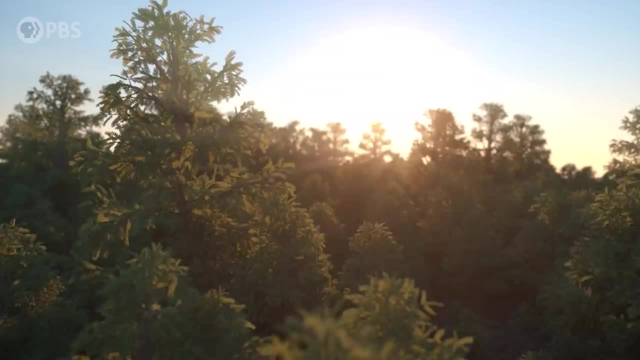 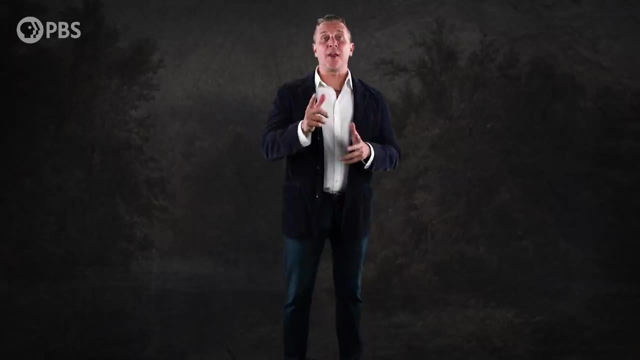 But it had both male and female spores, making it unique among its peers at the time. The female spores were bigger and contained a food supply for the embryo, So they're thought to be a precursor to seeds, And this helped Archaeopteris spread around the planet. 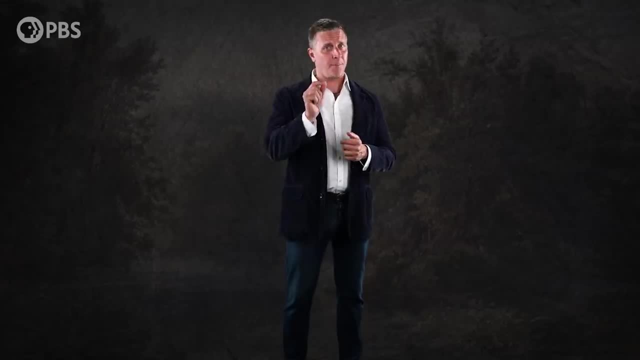 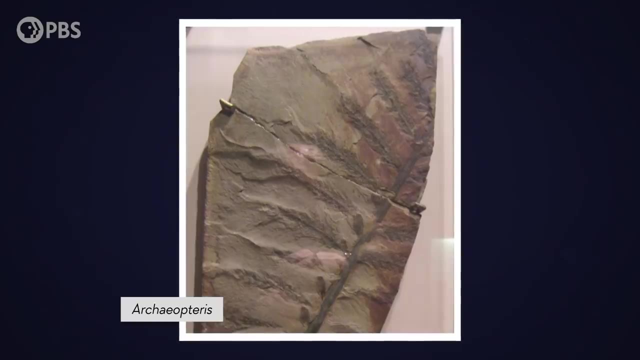 by making its reproduction even less dependent on perfect environmental conditions. Fossils of Archaeopteris have been found on every continent, including Antarctica. It's considered one of the earliest modern trees, appearing around 370 million years ago, And it could grow up to be 30 meters tall, which made it a giant of the Devonian forests. 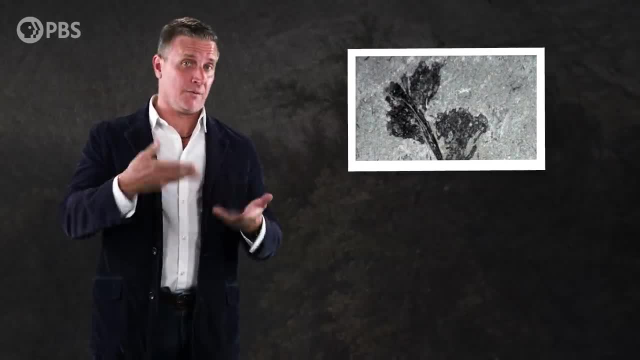 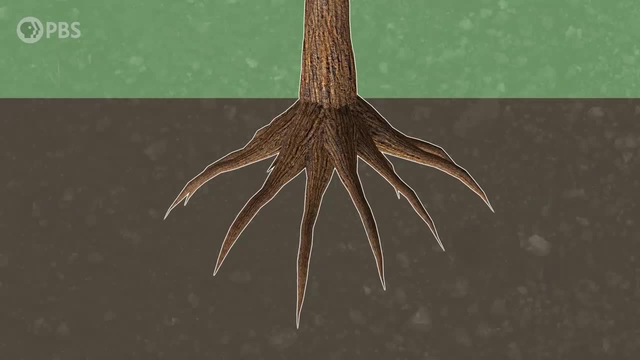 And, unlike those plants found at Gilboa that were originally mistaken for trees- even though they didn't have true woody tissue, Archaeopteris was full of the stuff. Their roots spread deep and wide, allowing for more effective collection of water and nutrients. 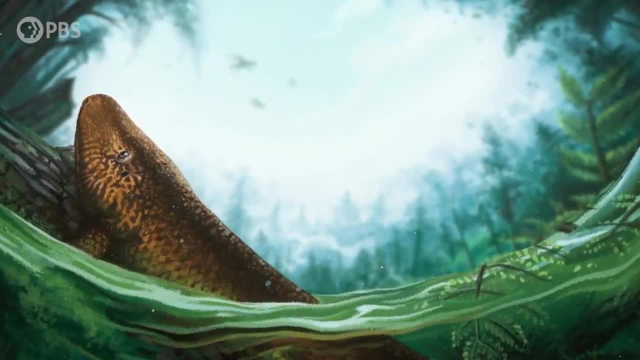 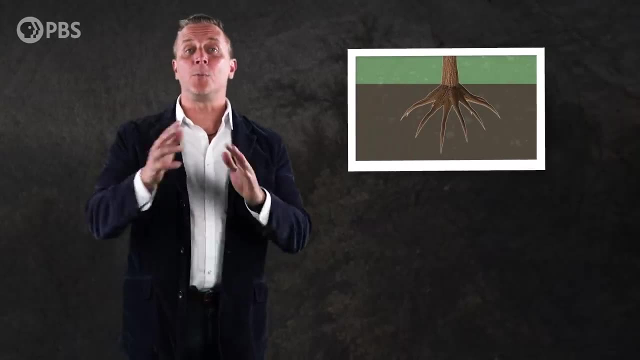 And Archaeopteris and other Devonian plants also created more habitats for animals and more food for them too, And their roots broke down rocks, releasing new minerals into bodies of water. At the same time, the root systems of all this vegetation created more stability in the sediment. 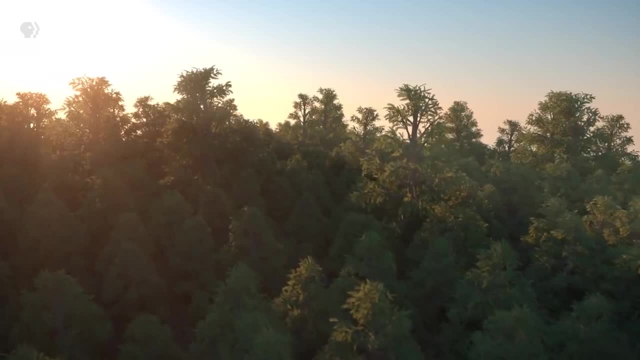 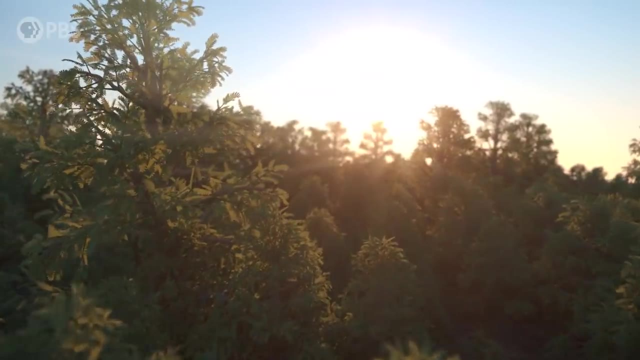 which allowed meandering rivers to form. The cycle of decay and renewal of these plants increased the amount of nutritious soil available, And the wood in these plants was directly responsible for a lot of the soil generation that took place in the Devonian forests. The organic component of soil called humus is mostly made up of broken down lignin. 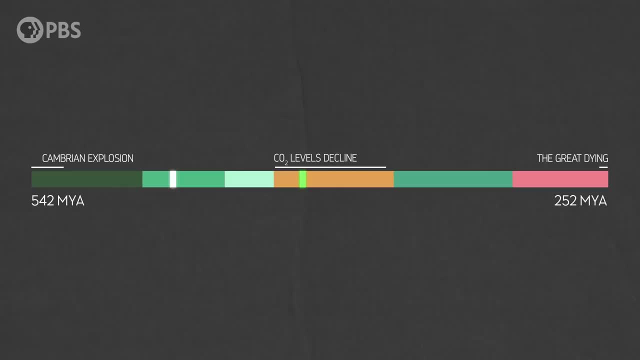 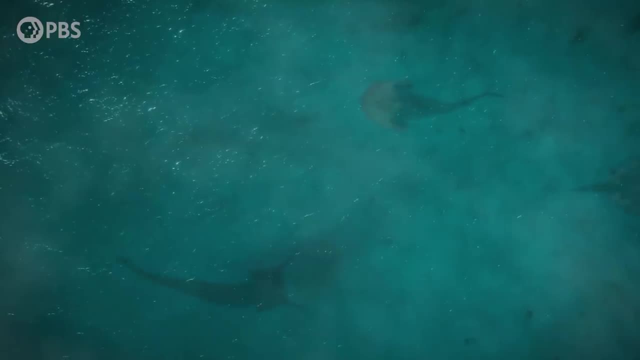 And between the weathering of rocks and the amount of carbon dioxide that the trees pulled out of the atmosphere, CO2 levels fell drastically from the beginning of the Devonian to the end. Now this, admittedly, was not great for a lot of the species living in the oceans at the time. 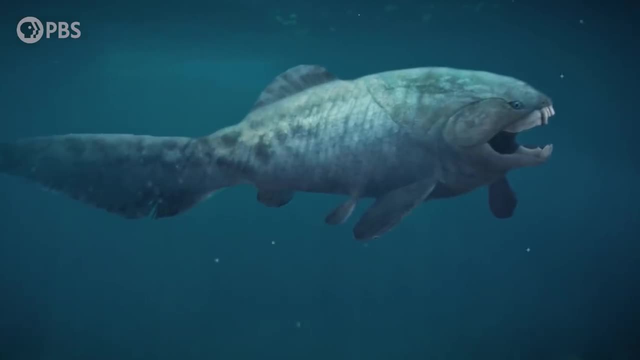 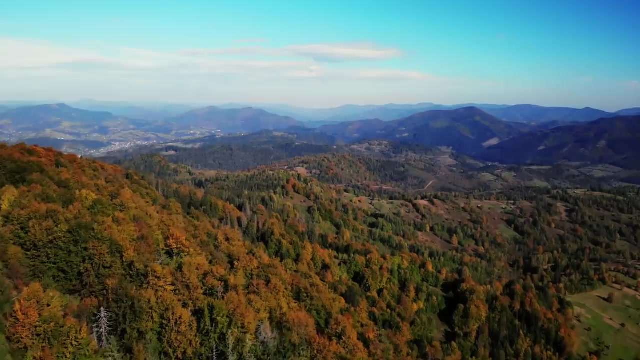 It was probably actually a major cause of the mass extinction that happened at the end of the Devonian, which really deserves its own episode. But the thing is, these trees directly created the world that we live in today, by changing both the atmosphere and the land. So while they helped end the world of the Devonian, if it wasn't for them our world might not have gotten started. By the end of the Devonian period, plants had developed almost all of the traits they would need to thrive. It would take another 200 million years for the next big plant innovation to appear: flowers. 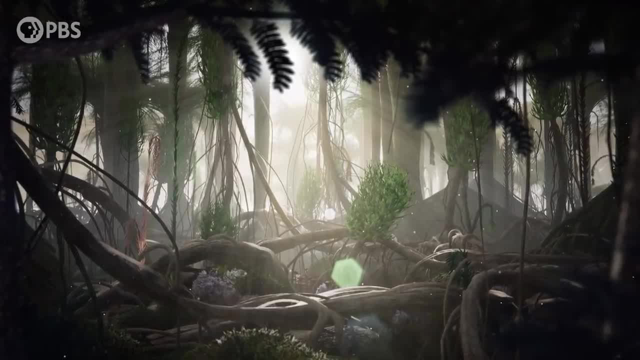 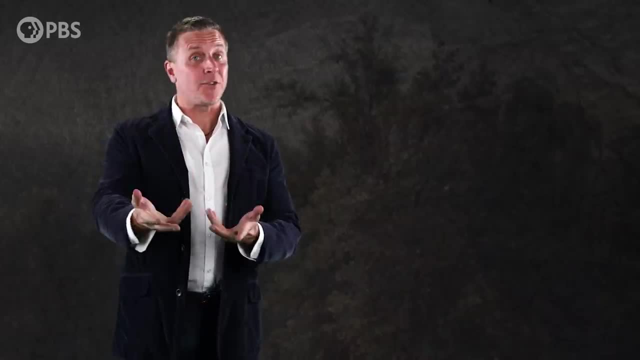 So, from the false trees of the Gilboa forest to the true trees like Archaeopteris, it's clear how big a difference the evolution of wood made in helping trees take over. And once plants were using seeds to reproduce, they had the handful of adaptations that made them mostly modern. 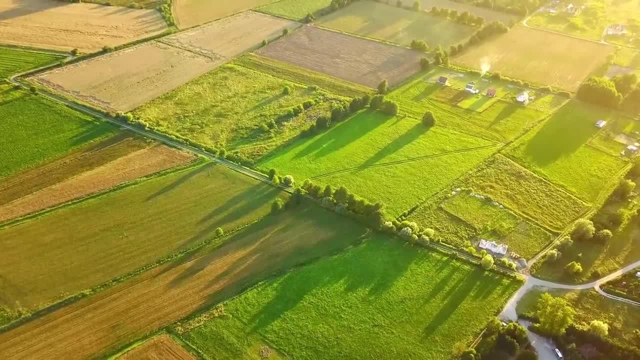 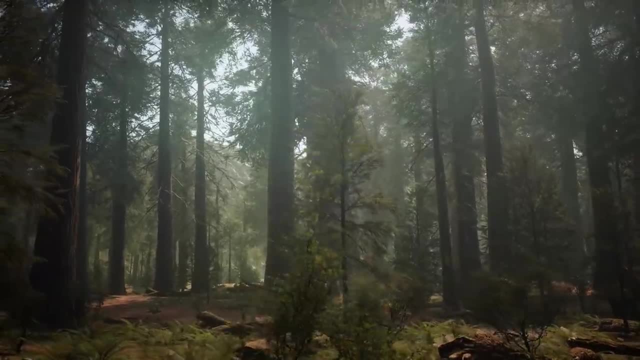 Roots, wood leaves and seeds. So while we might think that it's humans, or at least mammals, that have transformed the world the most, there's a chance we might not even be here if trees hadn't put in the work first.